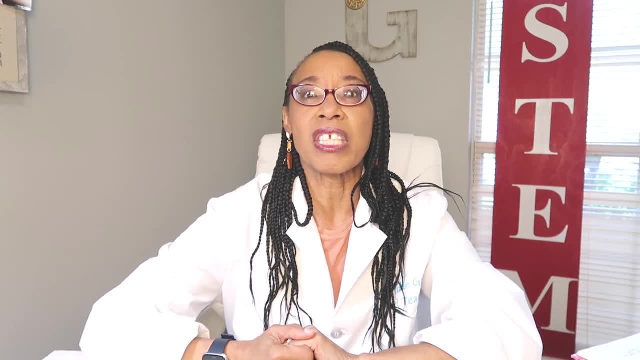 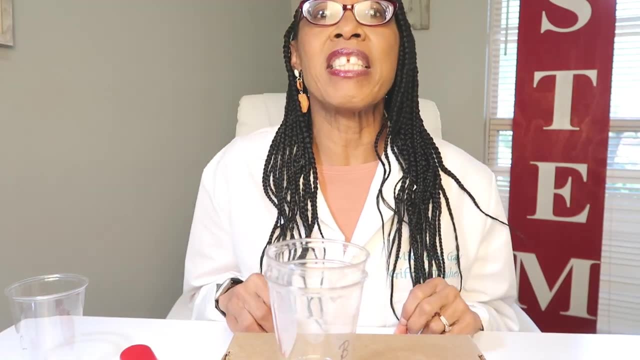 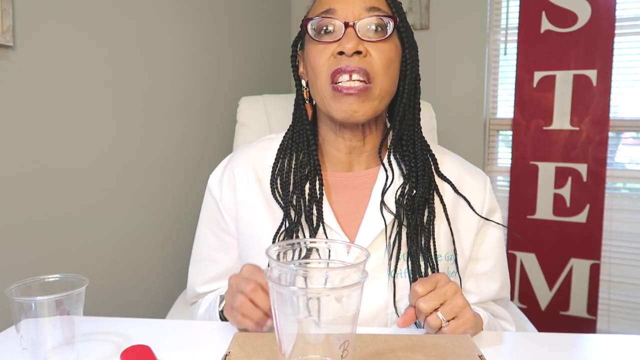 So we're looking at how does that heat energy, energy in motion, make those molecules move? I'm going to conduct two experiments: one on liquids and thermal energy and one on gas and thermal energy. Let's look at our first one. 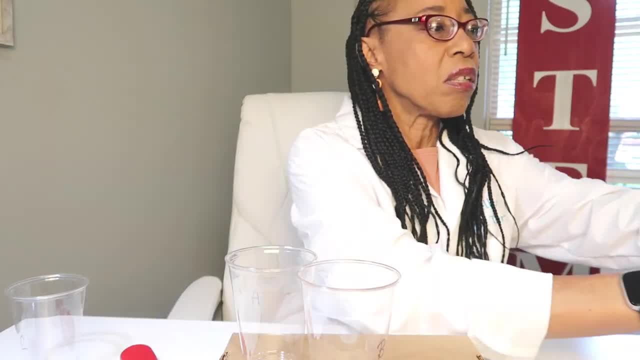 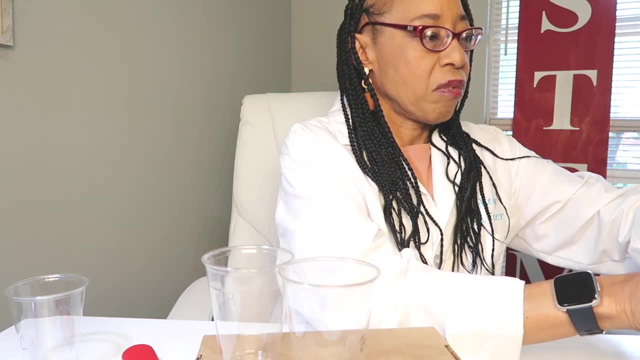 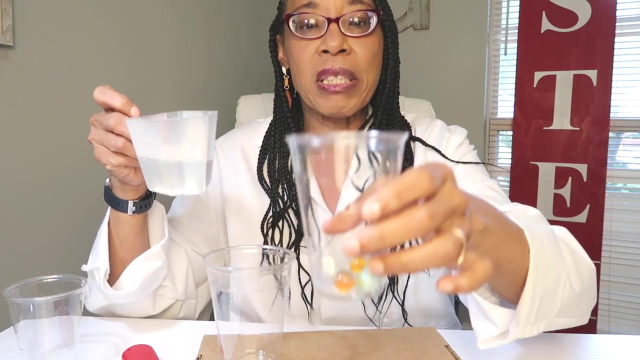 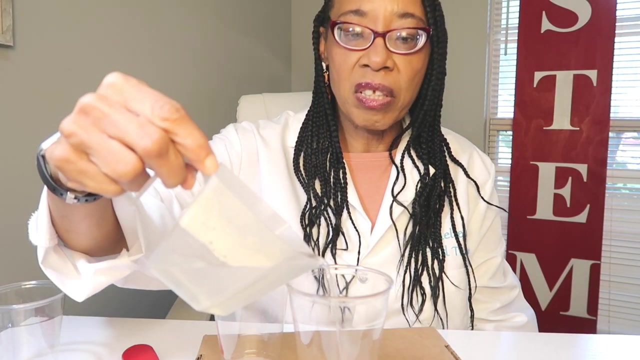 We're going to take some hot water and we want this water at boiling point. At the bottom of my cup I put some marbles and I'm going to keep those separated and I'm going to cover the marbles with hot water. 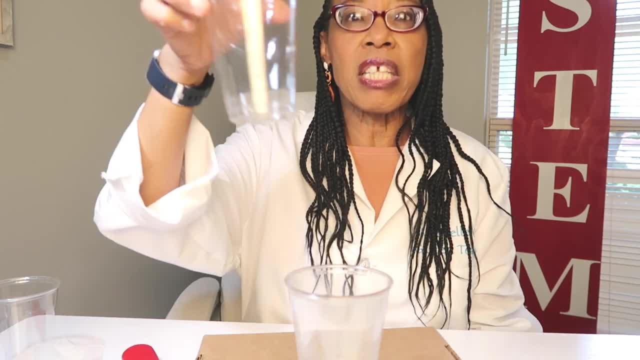 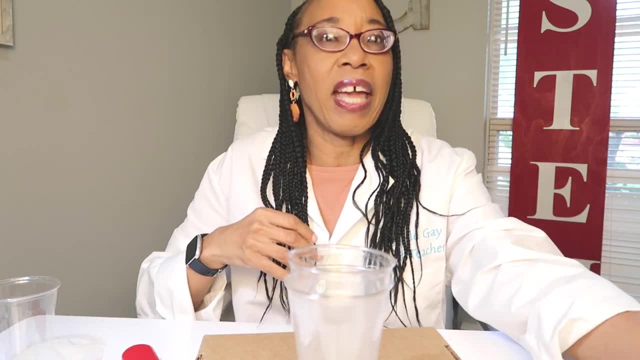 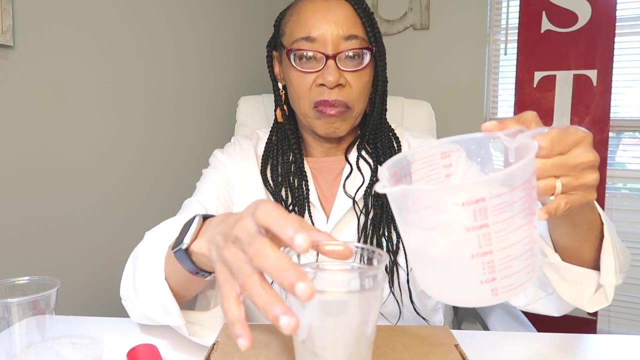 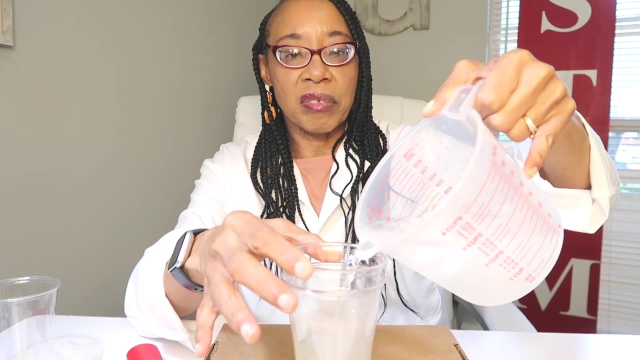 Now I'm going to insert another cup. This time I'm going to add cold water. I'm going to fill it to the top. I'm going to fill it to the top. I'm going to fill it to the top. 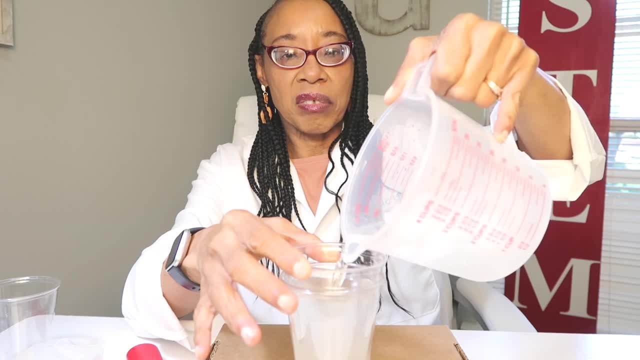 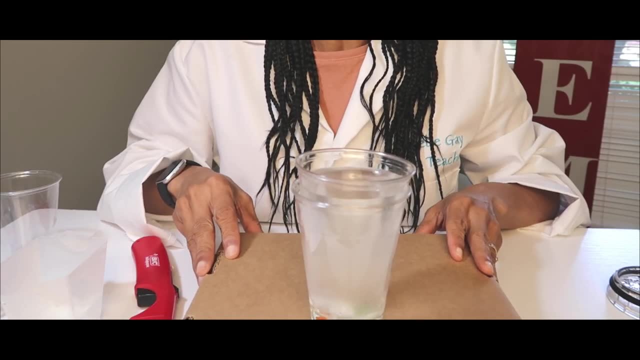 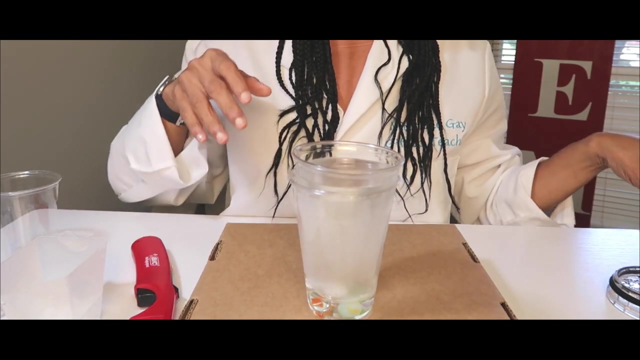 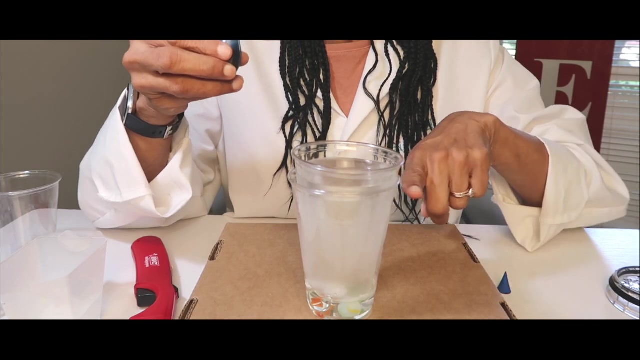 Now that we have our hot water at the bottom and the cold water at the top, we're going to add food color. I want you to carefully look and observe what occurs. 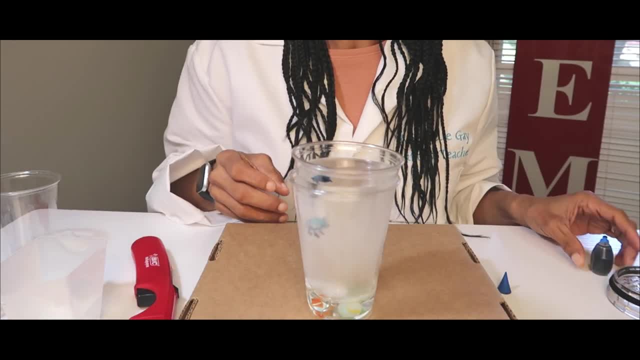 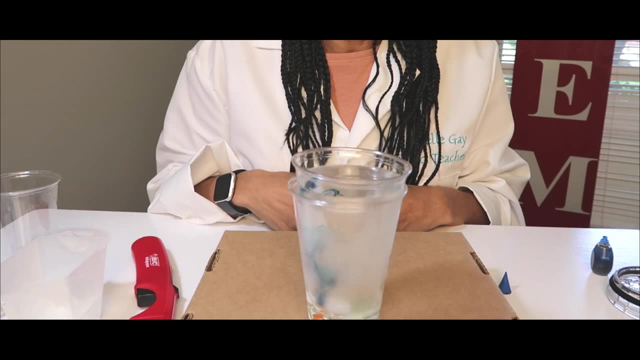 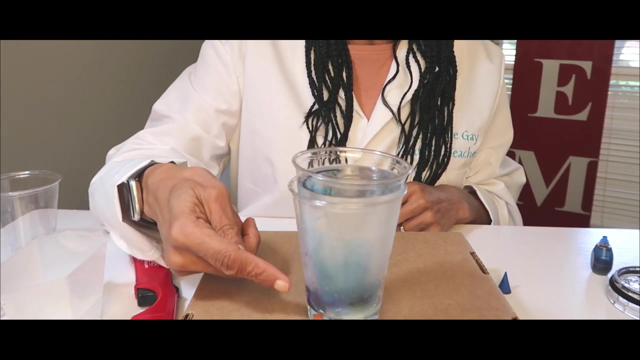 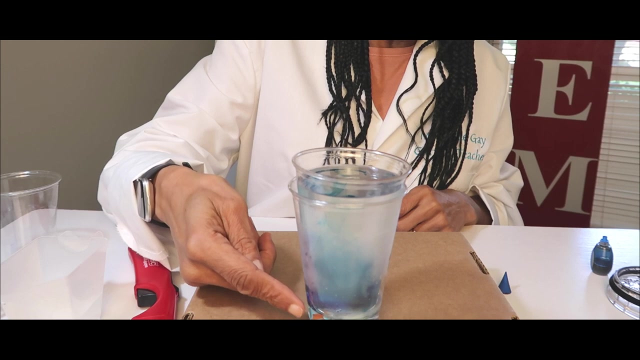 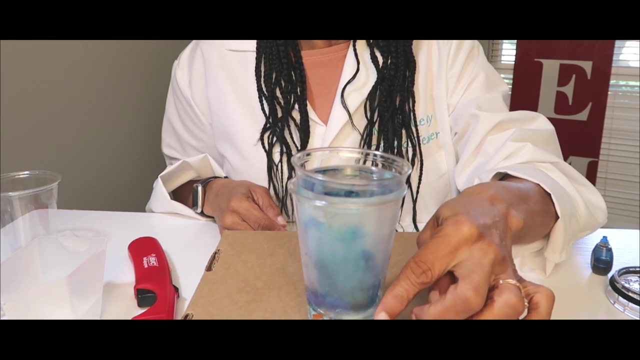 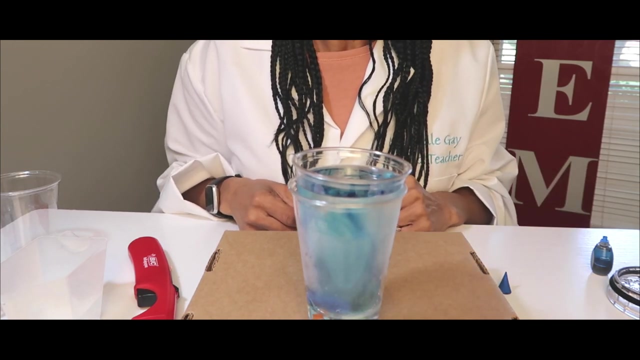 Notice the blue is at the bottom. At the bottom we have warm water now because of the hot water And because of that now, if you look over here, the blue is coming back to the top. That is because we call this convection. 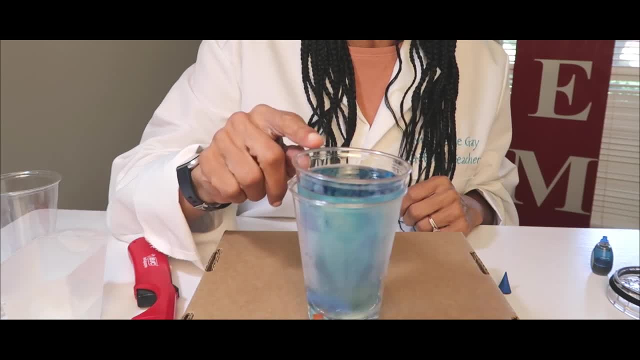 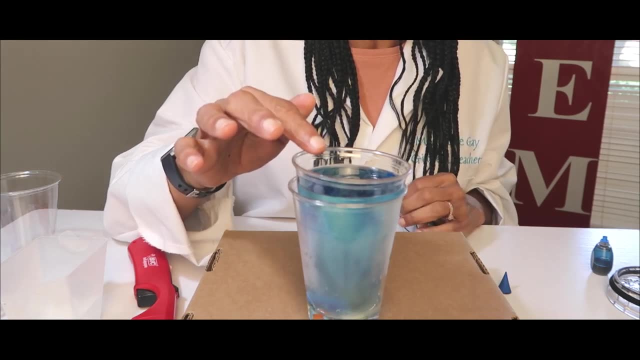 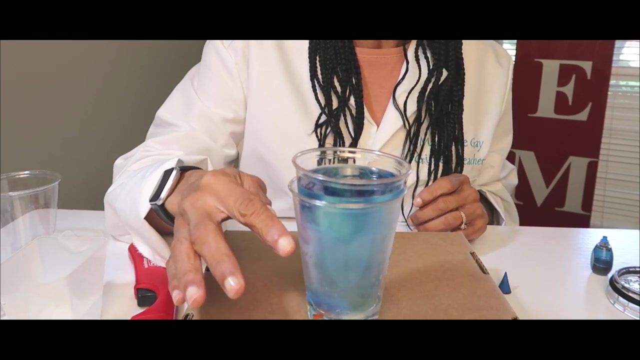 We have cold water at the top, meaning that we have less energy moving. And because this cold is at the top, the food coloring is denser And so it went to the bottom, floated to the bottom and then, because of the hot water, 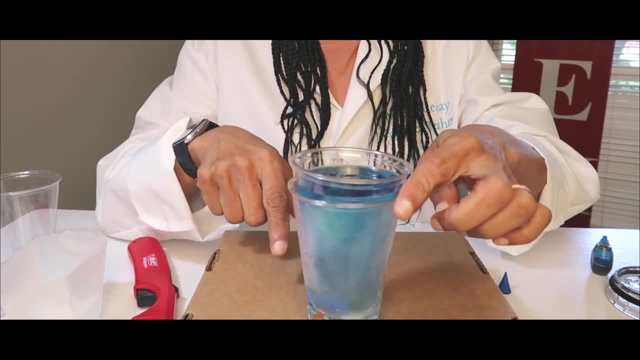 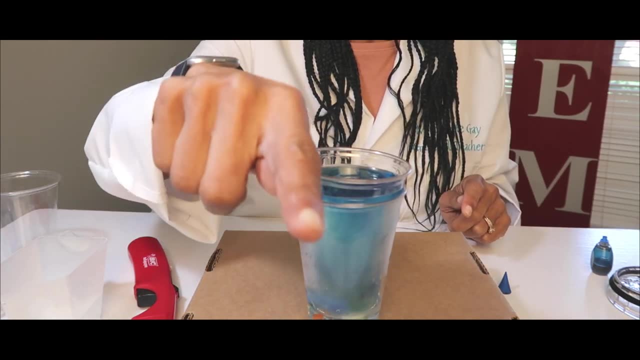 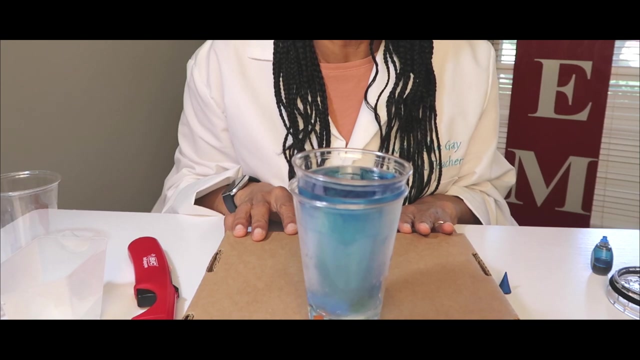 it began less dense and it rose back up because the cold became cooler. So we have this cycle of cold going down to the bottom of the warm and coming back up to the cold, And we call this convection. We're going to be looking at gas. 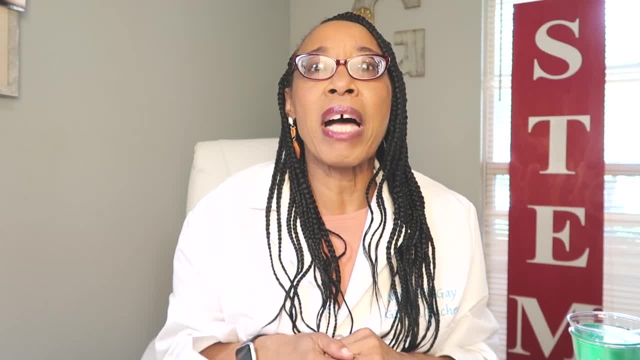 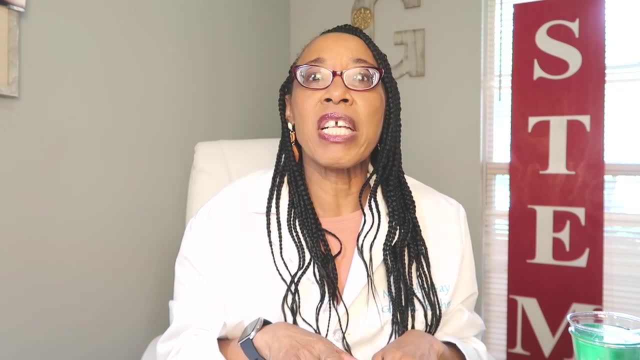 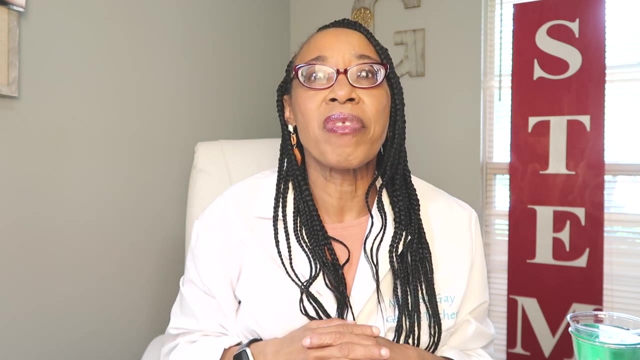 This process of convection is. when you think about your home, Have you ever observed that at the bottom of the floor is cooler compared to the area where the ceiling is? it's warmer. Well, that's what we're going to look at. 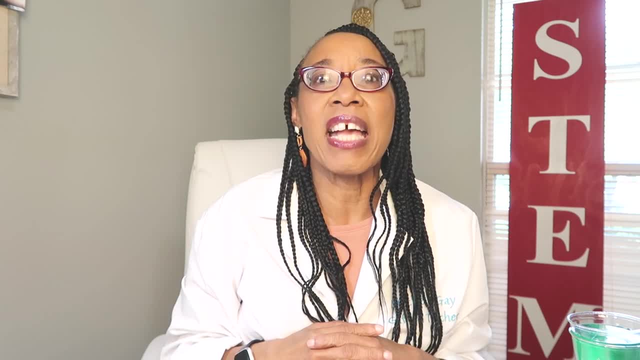 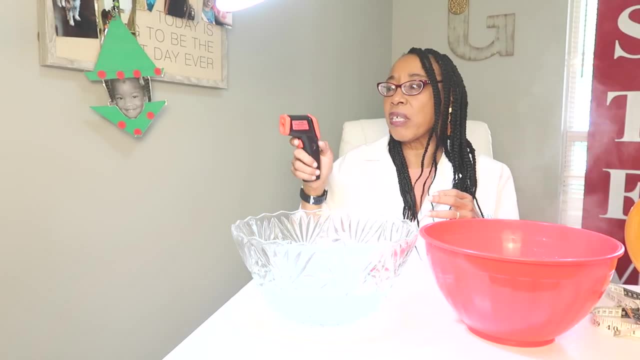 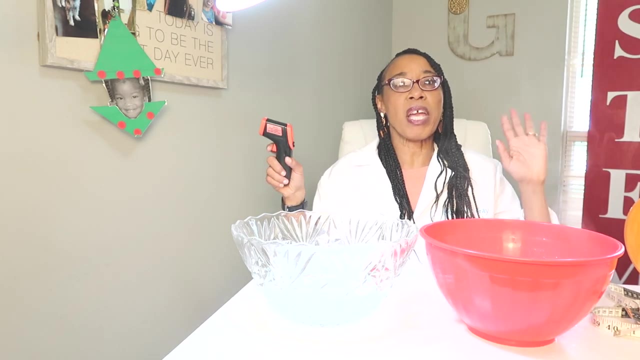 How does convection work? Convection affects gas, gas, the air we breathe. Let's take a look. I have my thermometer and remember I told you that it's cooler at the bottom of your home, near the floor, compared to the top of the home. 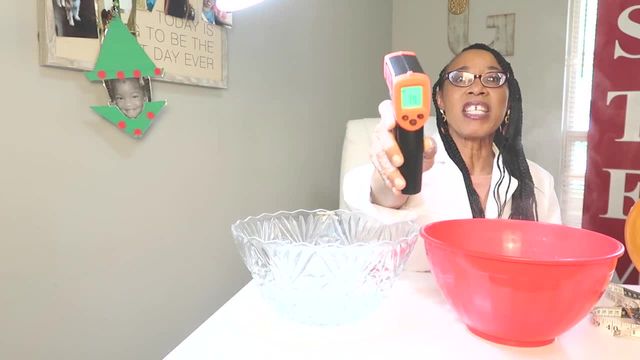 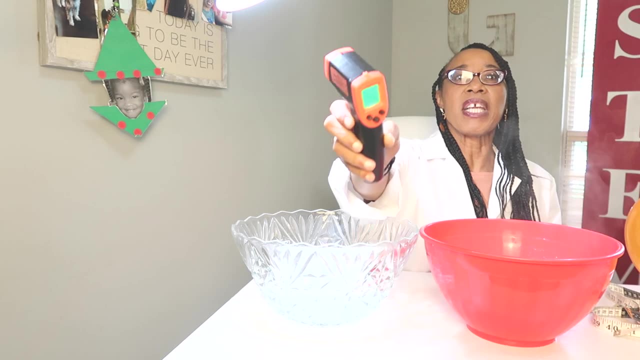 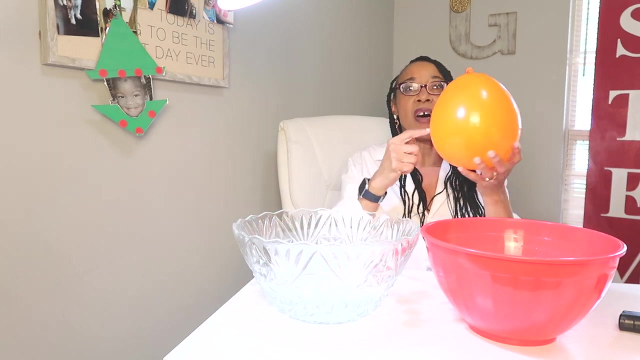 So I just took the temperature and it reads 79 degrees for the top. Let me check the floor. Let's see It reads 73 degrees. I'm going to measure the circumference, meaning all the way around, Woops, Okay. 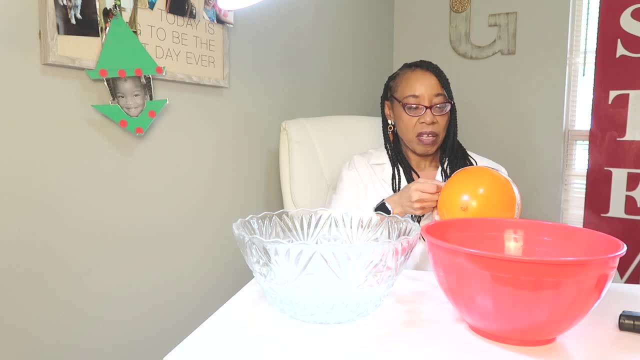 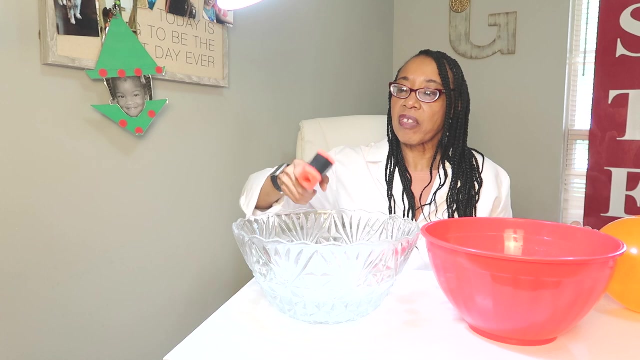 I have my thermometer Now. Okay, Okay, have 52 centimeters. Now I'm going to take the balloon and submerge it in this cold water. Before I do this, I do need to take the temperature of the water. It says 37 degrees- Pretty cold. 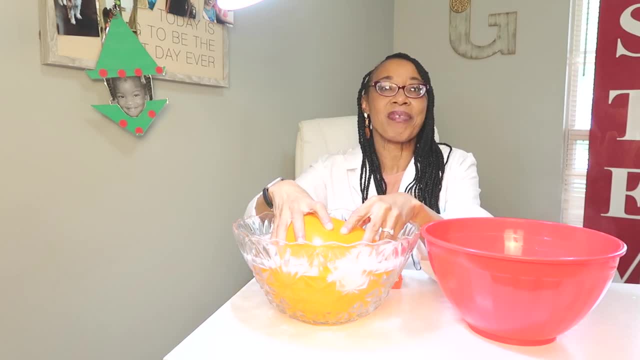 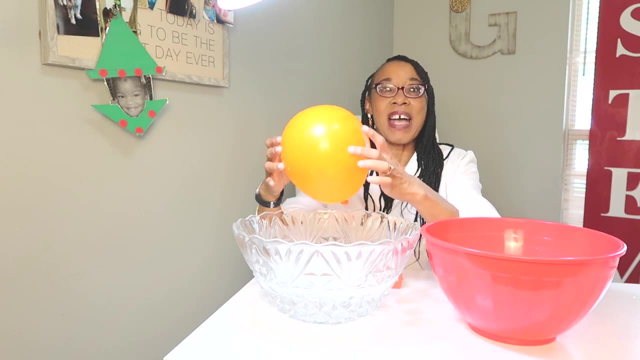 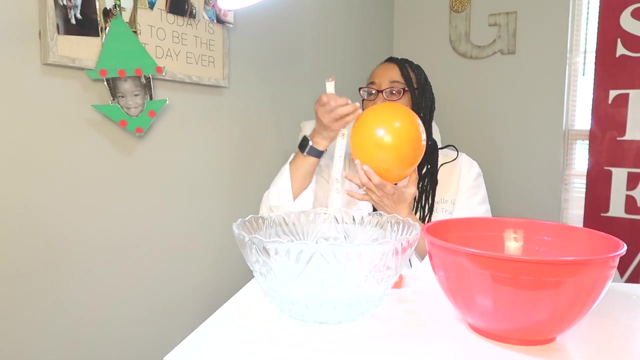 I'm going to submerge it for one minute. I'll be back. All right, Let's take another measurement. I dropped my tape measure. Let's see. Remember, the first one was 51.. Let's see if we have anything different. 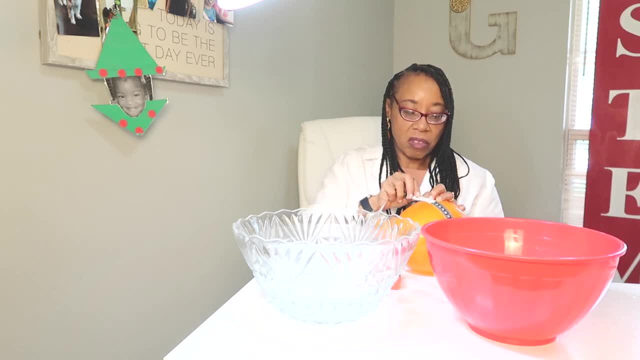 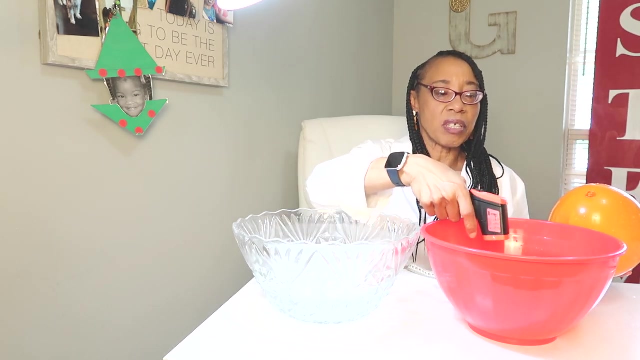 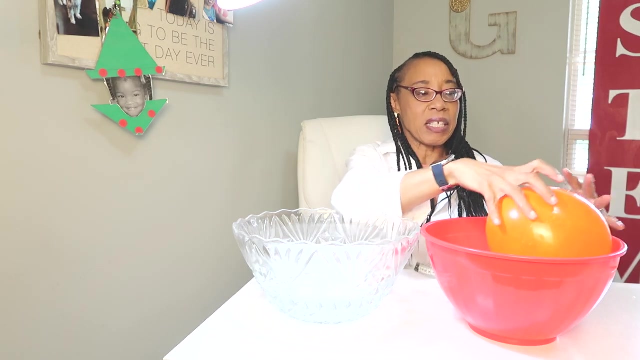 This time it's 52.. It went up some. All right, Now we're going to submerge it in the hot water. Let's see the temperature. This is 125.. We're going to submerge it for a minute. All right, Let's measure. 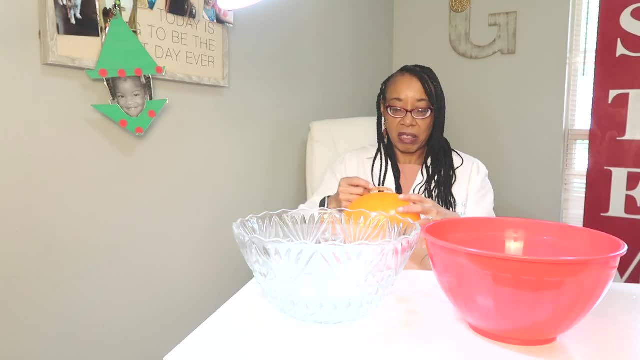 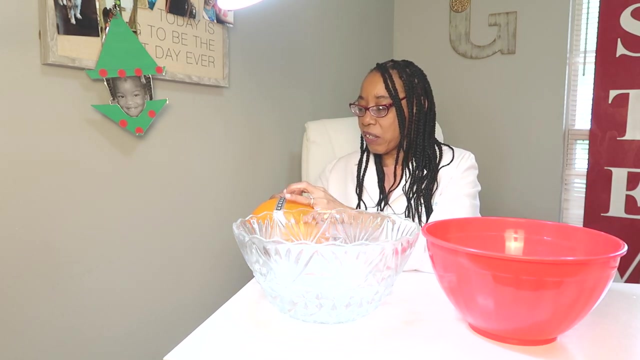 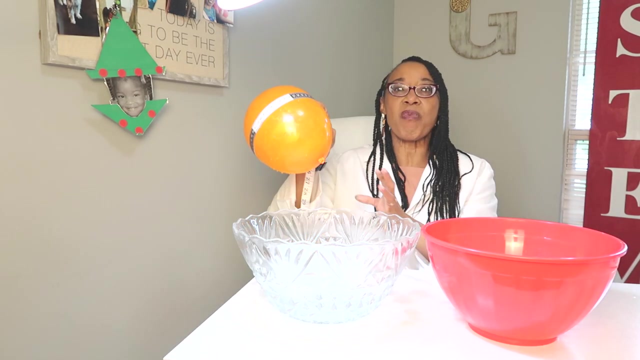 Let's see what we get this time. This time we have 54. 54. So it expanded. It got bigger because of the heat. Well, let's test again and see what happens in the cold. What do you think? Just looking at it, do you think it shrunk, Or did it get bigger? Guess what? It went back down to 51 and a half. 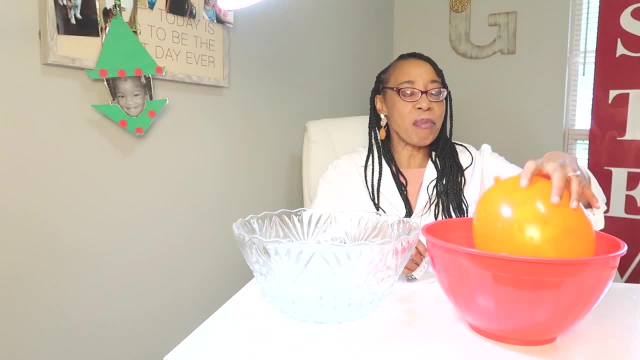 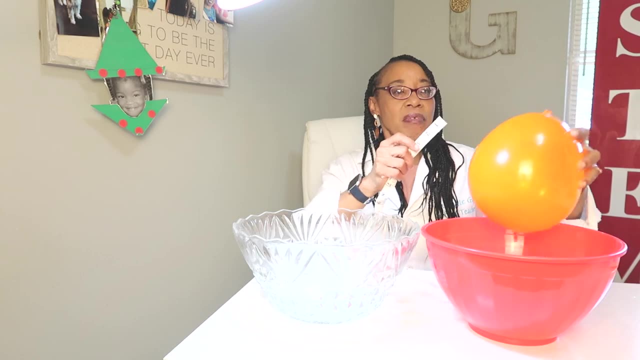 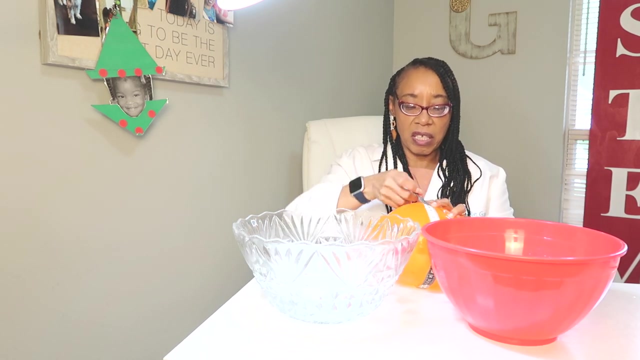 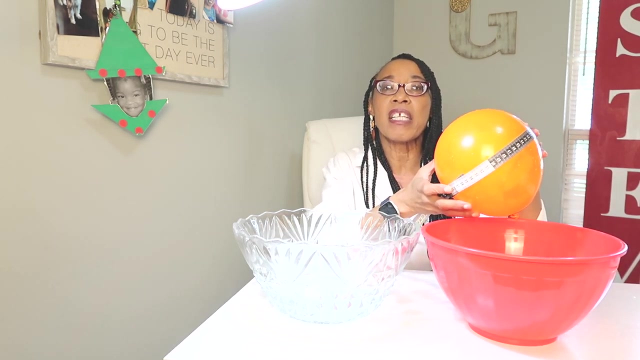 51 and a half, And one more time in the hot water for a minute. Okay, Let's measure. Do you think it expanded Or did it shrink? It expanded again to 54 and a half centimeters. So what does that tell us about heat energy? 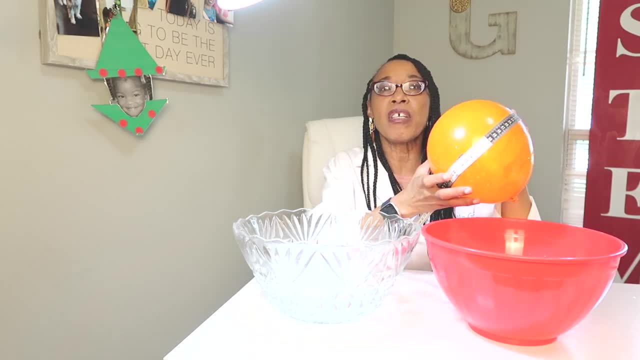 One. we know that the molecules are moving faster with the air inside the balloon when it is what Hotter Compared to when it's colder, And we can see this because the balloon expands. Anytime there's a solid liquid or gas and it is affected by heat energy, it expands.